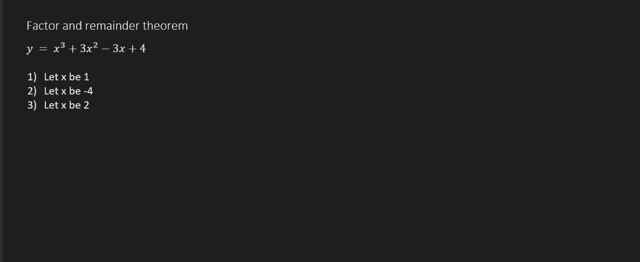 over here and let x be 1.. So just plug 1 into that. and what would you get? Well, if we go plug 1 in, you're going to get an answer of 5.. So what does that mean? It means that the number x equals. 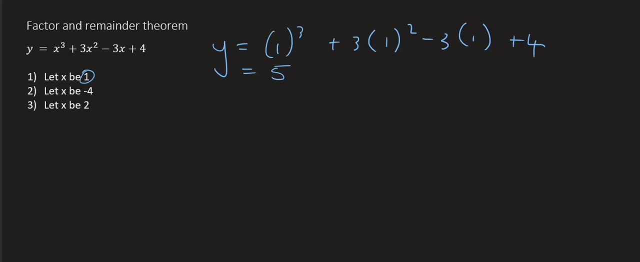 to 1 is not a factor and the remainder is 5.. So in a test they could either ask you to see if x equals to 1 is a factor, or they could ask you in the bracket form. So they would give you the expression and then they would say: is x minus 1 a factor? and then they would say of, and then 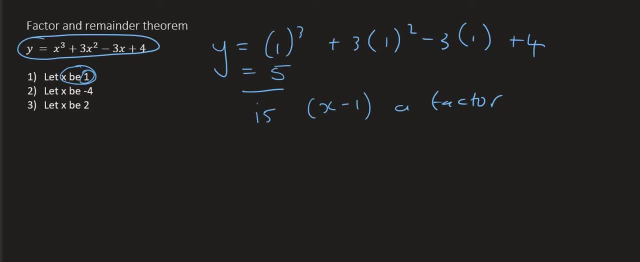 they would give you this equation over here. So they would say: is x minus 1 a factor? and then they would say: is x minus 1 a factor? and then they would say: is x minus 1 a factor? and then. So remember, when they give you the bracket form, then you must always do the opposite. So if it, 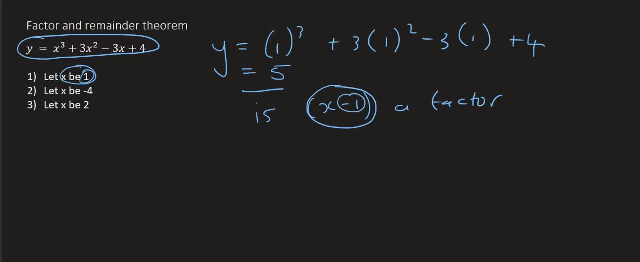 says minus 1 over here, then you must plug 1 into the equation. So nonetheless, the number 1 is not a factor of that expression and the remainder is 5.. We're now going to plug minus 4 into that expression, and when you do that you're going to get an answer of 0.. So what that means is that. 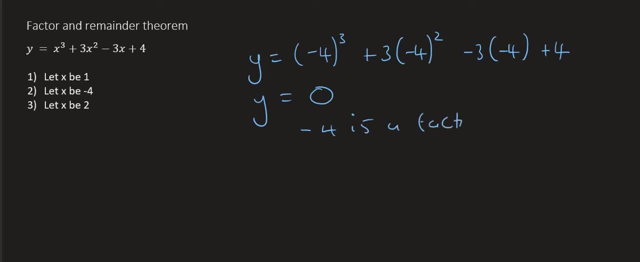 minus 4 is a factor. So when you get an answer of 0, you're going to get a factor of x minus 1.. So when you get an answer of 0, it means that it is a factor. In a test they might say is the: 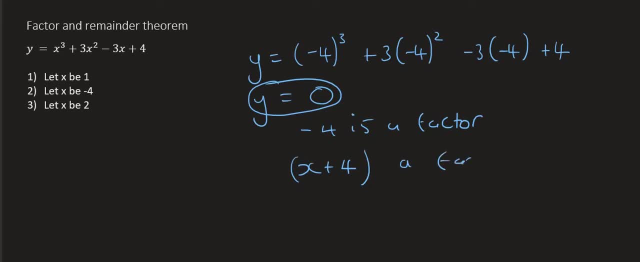 expression x plus 4 a factor, Then remember the opposite of x plus 4 is minus 4.. So you'd plug minus 4 into the equation. If you get an answer of 0, then it is a factor. I mean, I've seen some. 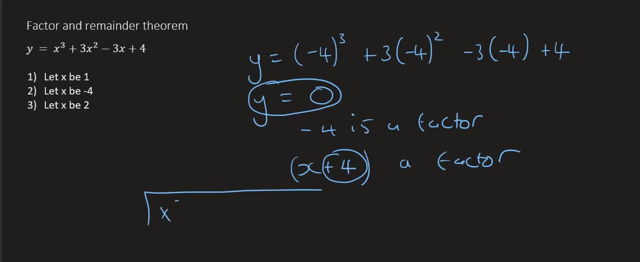 teachers show this using long division. So they would do something like x3 plus 3x squared minus 3x plus 4, and then they would put x plus 4 into the equation. So if you get an answer of 0, then you. 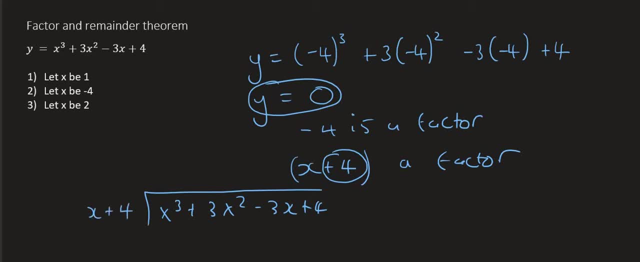 get x plus 4 over here, and then they'll do division and they'll see if you get a remainder or not. I mean, that is mathematically correct, but it's overly complicated. Then, lastly, we're going to let x equal 2, and when you do that, you're going to get an answer of 18.. What that means is: